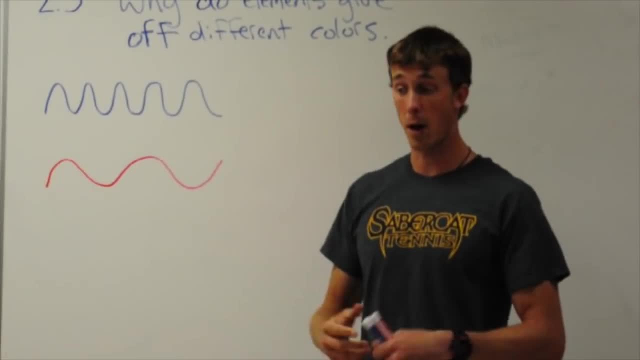 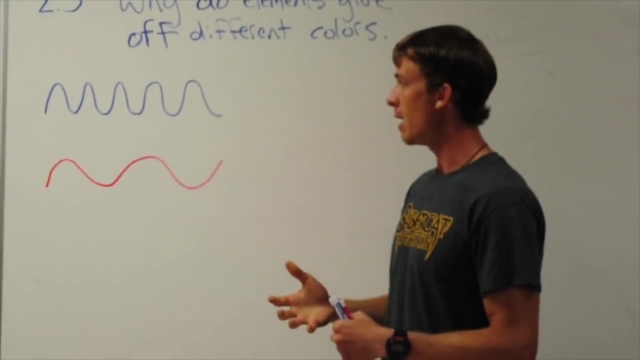 roast a marshmallow versus a s'more. to make a s'more And I want you to like, if you want to cook it really fast, so the s'more that you're trying to make, you have to do it really quickly. So what flame in the fire would you want? Because there's red and blue. 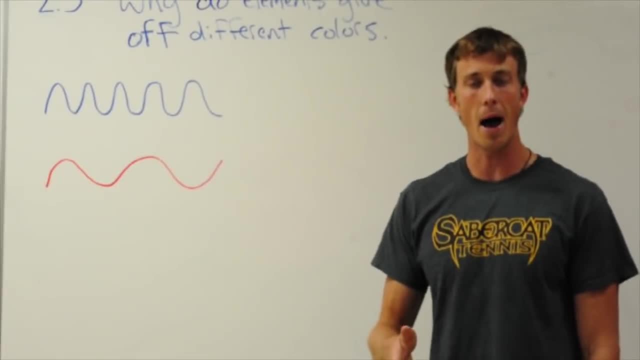 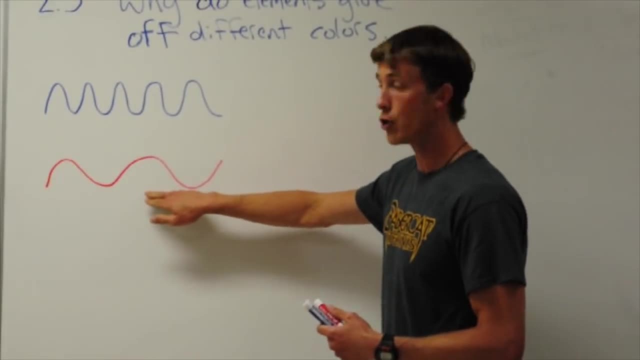 And I think you naturally kind of know that the blue flame is a lot hotter, So you can cook your marshmallow and have your s'more a lot faster. So the idea is, this is going to be low energy and this is going to be high energy. okay, So that's important to 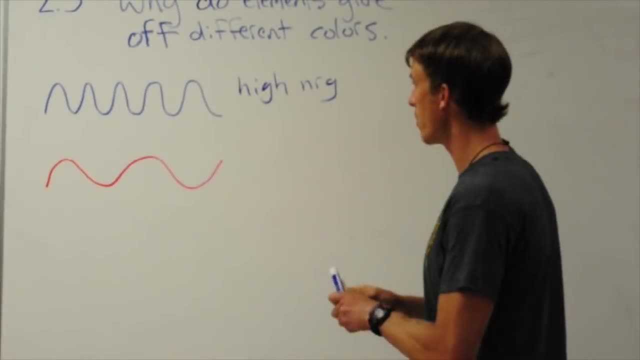 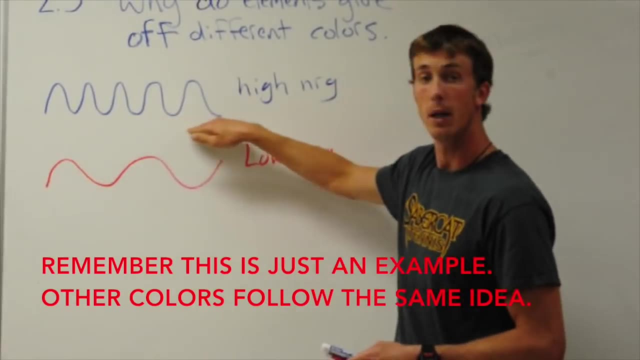 understand. So I'll put NRG as energy, just as an abbreviation. This is low energy, All right, so the whole idea here is that the higher the frequency, the more energy. The lower the frequency, the lower energy. So colors are related to energy in a way all. 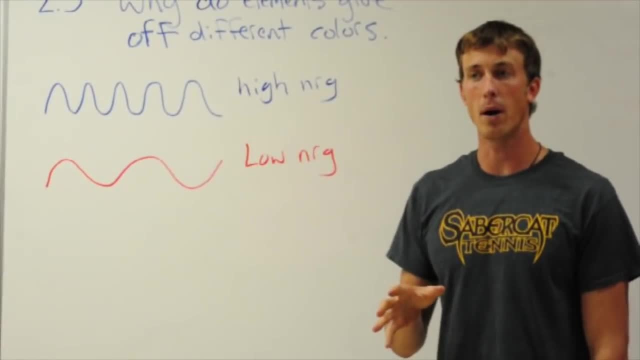 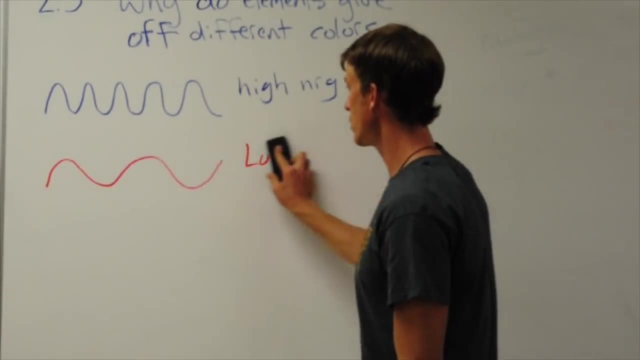 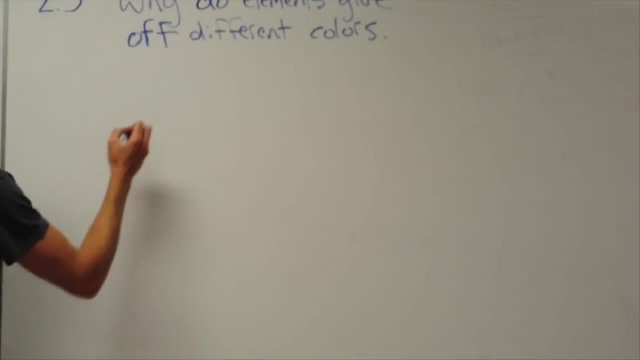 right. So when you give an element more energy, it's going to emit a higher frequency. All right, so that's kind of just the basics of it. Now let's get into how it would look of an element. all right, So I'm going to just draw a. it's called a Bohr diagram. I 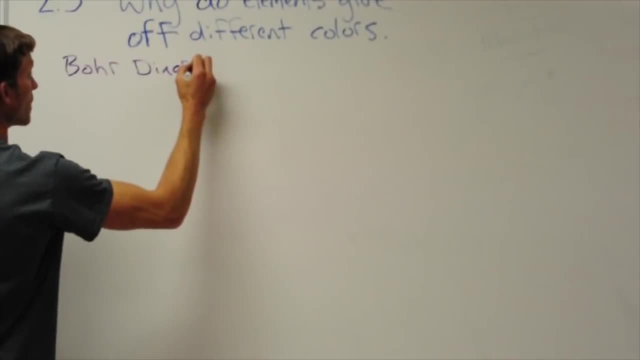 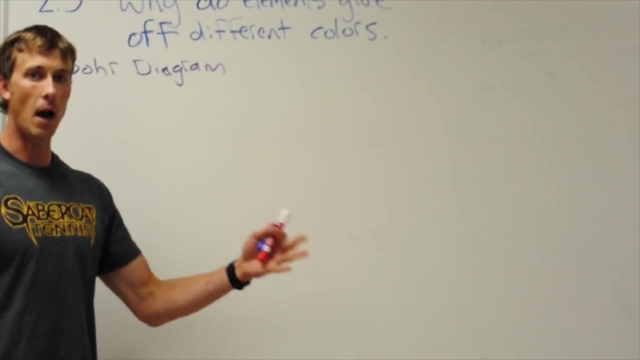 guess I'll write that down All right, so you can look this up if you would like. but this is a simplified version of. this is a simplified version of an element of like how electrons are in an element in an atom. I should say: okay, So in an atom. 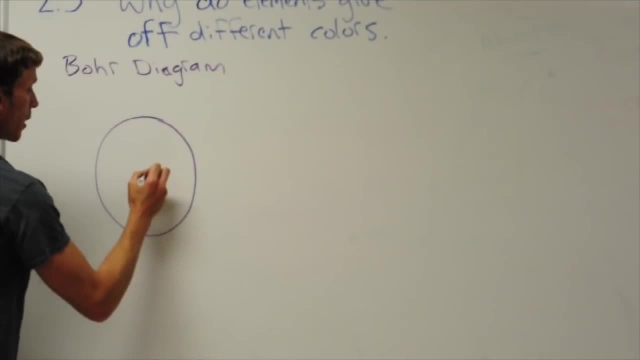 you know you have your protons in the middle and you have your neutrons, but we're not really worried about that. okay, We're more. there's more about it where there's energy levels. So let's just say we're right here, and I'm going to fill this in as that's the 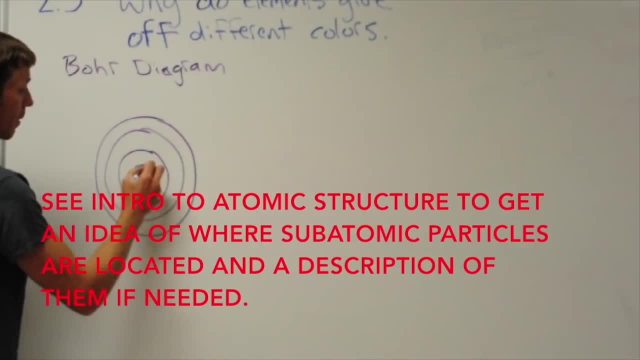 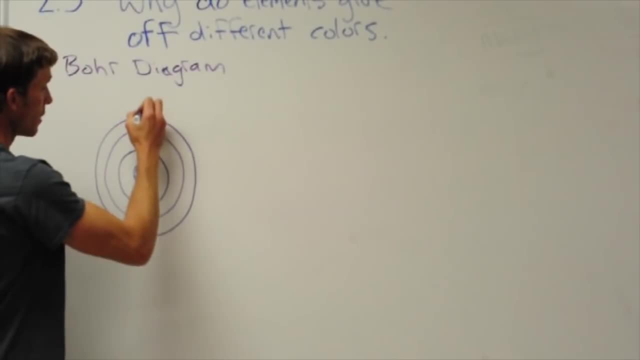 core, where the protons and neutrons are okay. So we're not really worried about that part, but we have let's. for this example, we have one energy level, two energy levels and three energy levels. So this has three energy levels. 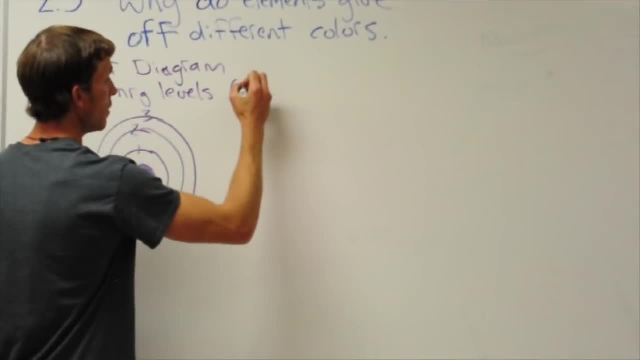 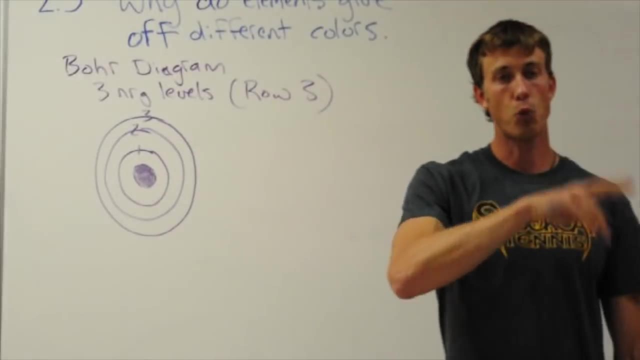 Okay, that must mean, by the way, it's in row three of the periodic table, and we'll get into all of that a little bit later, but just a side note: each row indicates how many energy levels that atom has. Periodic table is really cool, and your next unit you're. 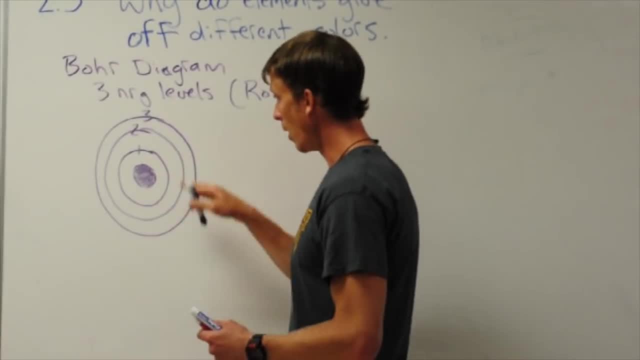 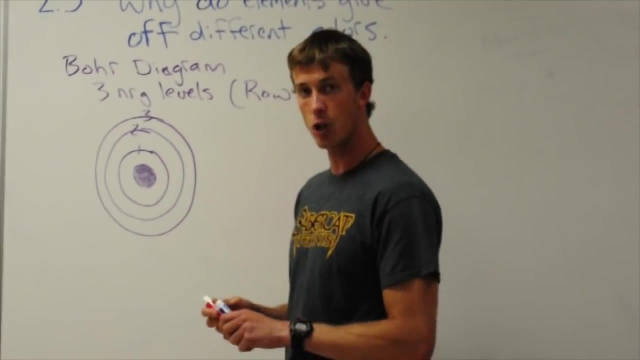 going to get into that a little bit more, but there's three energy levels. Electrons go in these. all right, Each energy level has a certain amount of electrons that can fit. The first energy level could have two, so I'm just going to put an electron there. 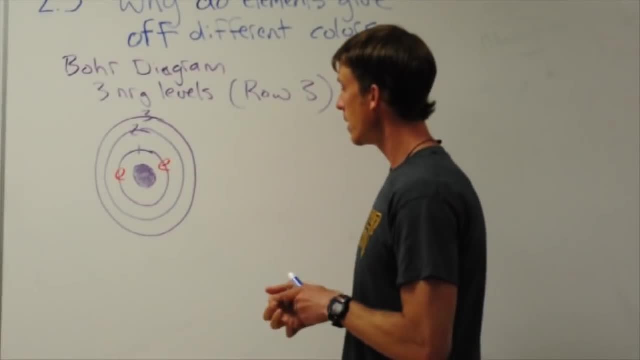 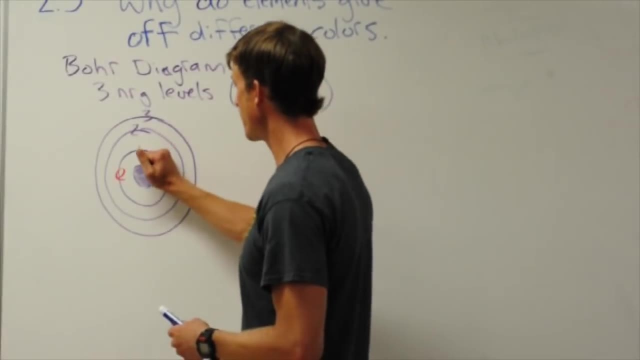 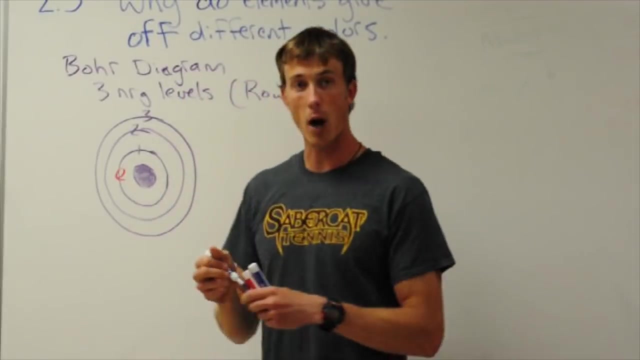 an electron there, okay, And I'm going to just leave it there. So it has two electrons. so we're looking at helium, okay. In fact, let's just make it even simpler and let's just focus on hydrogen. okay, So hydrogen has one electron and that electron can move. 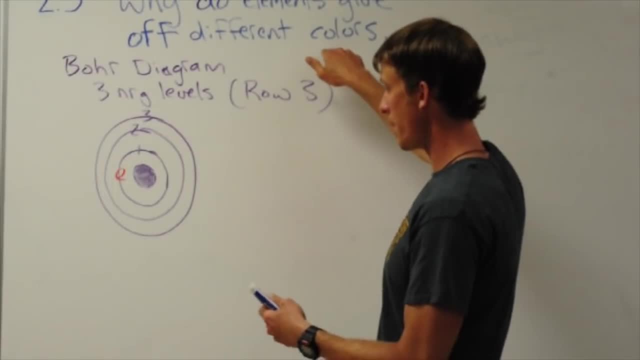 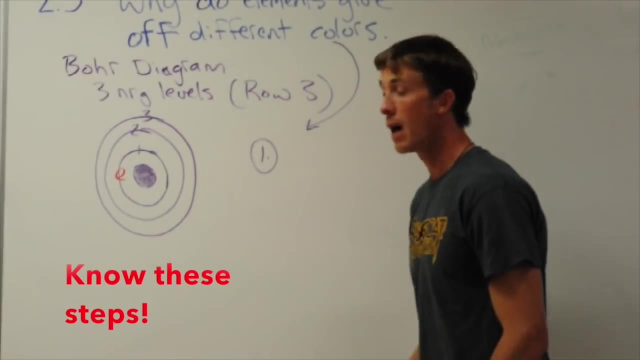 all right. So the first thing on how light, how you can make a color, so I might make a little note here of color, how it actually happens. So number one: I'm going to add energy. all right, So I'm going to add energy to the atom. 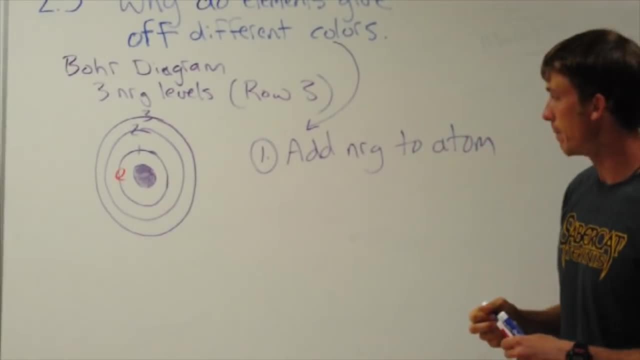 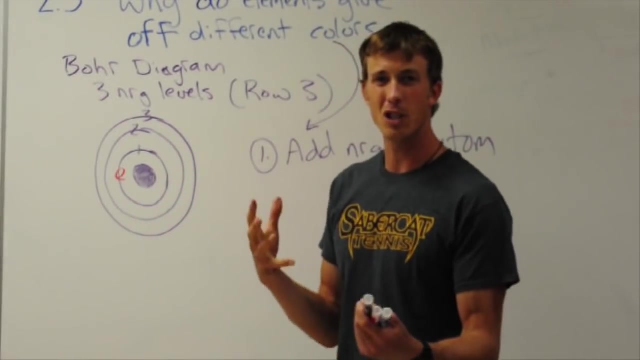 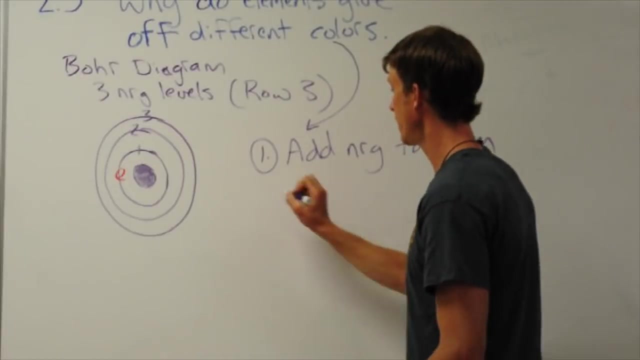 I'm going to add energy to the atom. So basically I'm going to add a photon- it's called- or some sort of energy, and photons are just packets of energy, there's just a name for it. and you hit this electron with energy, it gets excited, okay. So the electron gets. 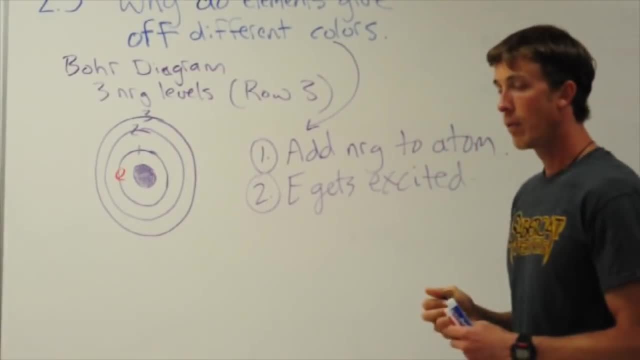 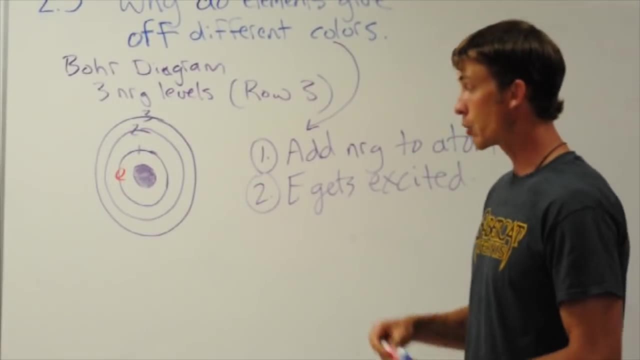 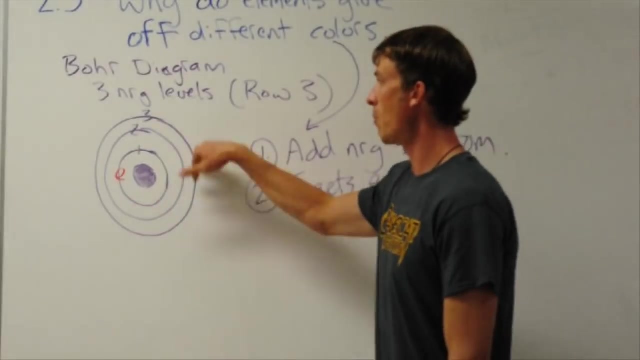 excited. When it gets excited, it's like having Mountain Dew or something like that, where it has a lot of caffeine and it wants to move. So it's going to move. now, all right, Depending on how much energy you put into. it depends on how many energy levels it moves Now there. 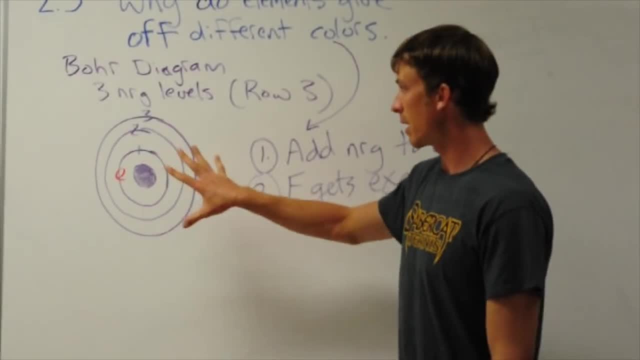 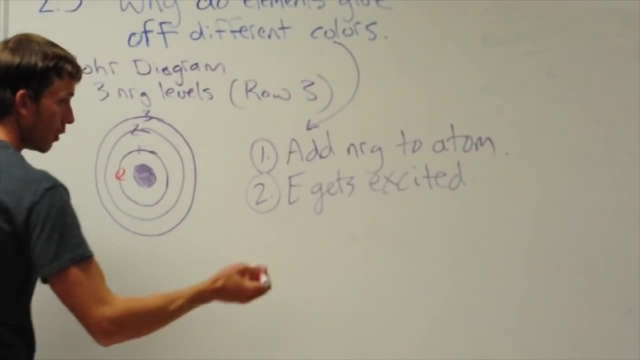 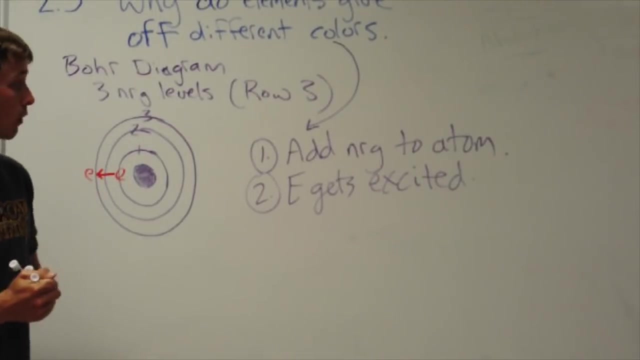 are more energy levels available for every atom. but I'm going to simplify and put two more than the one that this electron is in. Let's just say it goes into energy level number two, So it's going to move here. So now the electron is at energy level 2.. 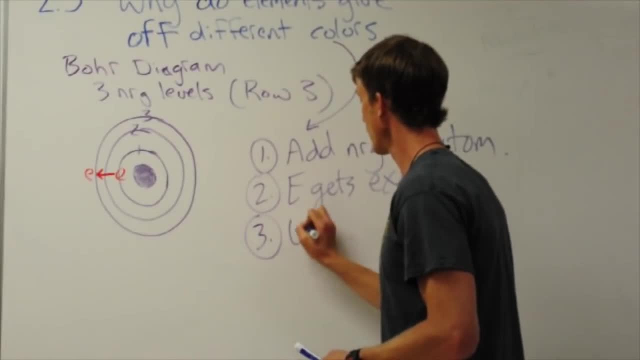 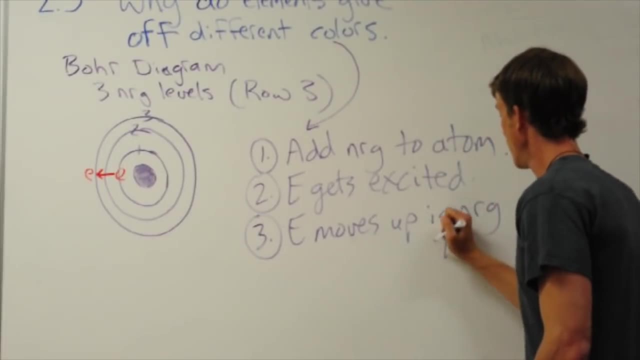 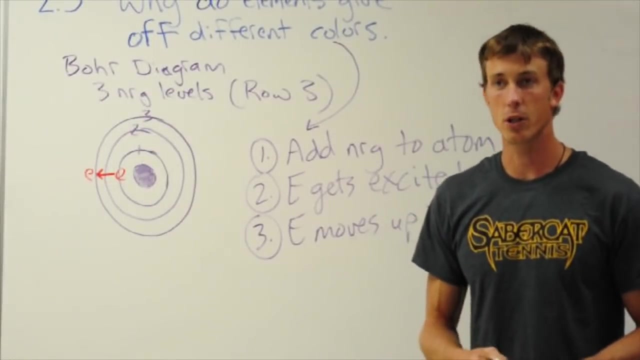 So that's the next step. So the electron moves up in energy levels. So after it moves up in energy levels, it runs out of energy, just like if you had a Red Bull or something or Mountain Dew: you're going to run out of energy. 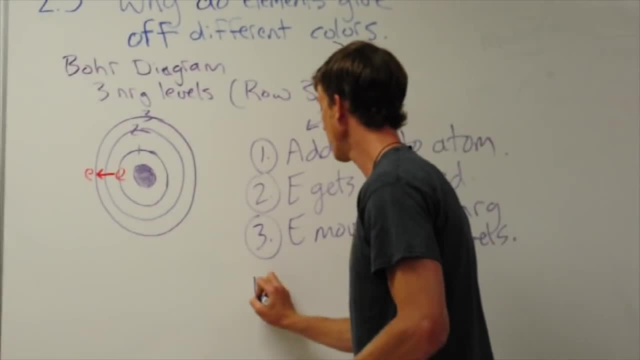 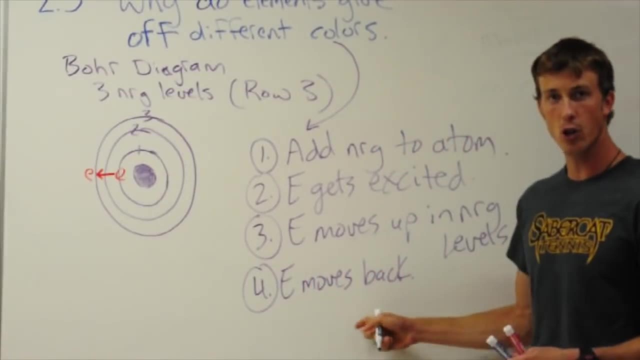 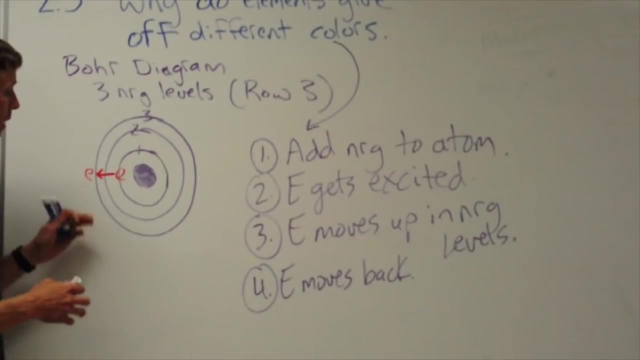 So that electron goes back, So electron moves back. electron moves back, So it moves back to the original position. So I'm going to draw that, But as it does, it goes back and it emits light. So let's just say that this is not very high energy. 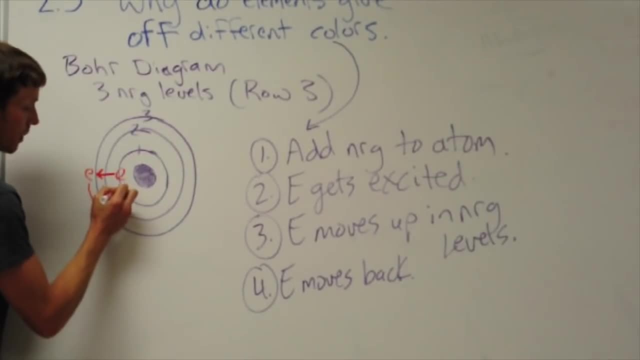 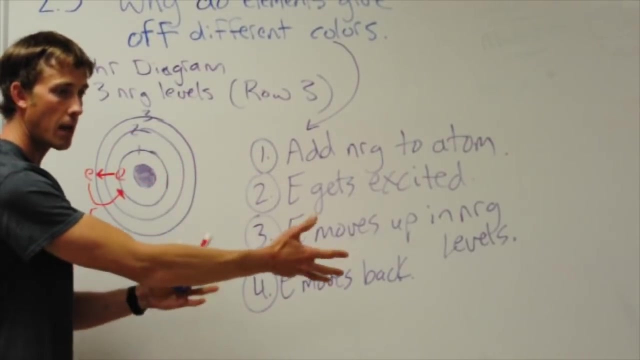 So the electron goes back to the original spot, But now, as it does, it emits light. Light Because if it's at high energy and it's going to low energy, there's a difference of energy now. So the energy has to leave. 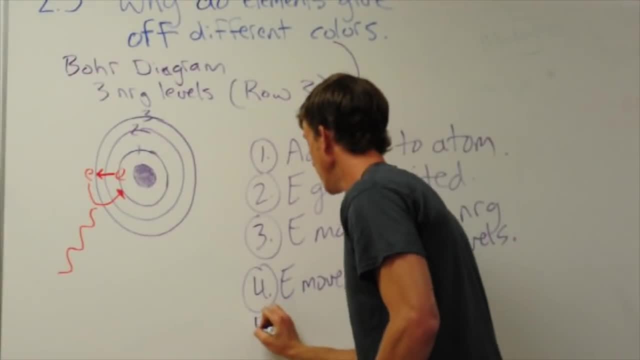 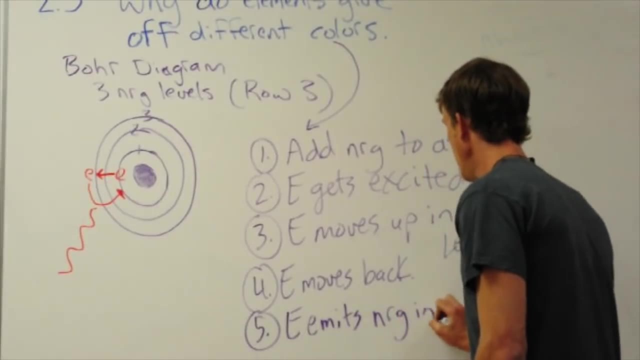 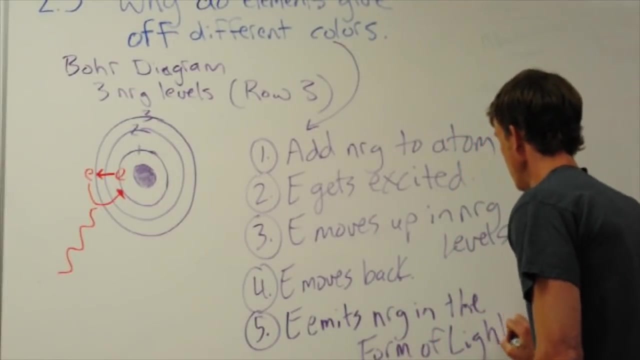 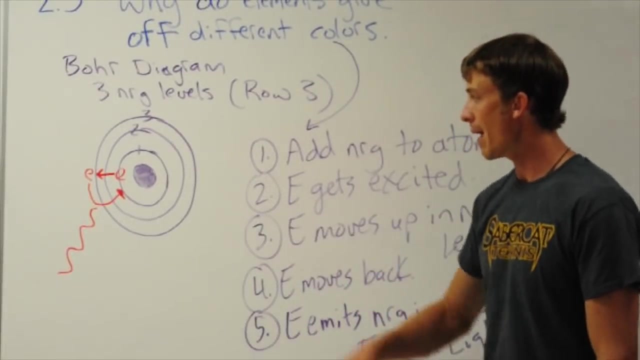 And it goes in the form of light. So the last step basically, is: the electron emits energy in the form of light. So that is it. That is energy, Light is energy. So you can see that if it emits red, the electron did not move that far up in the energy levels. 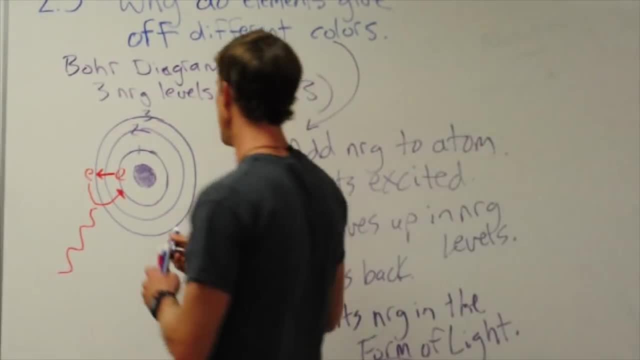 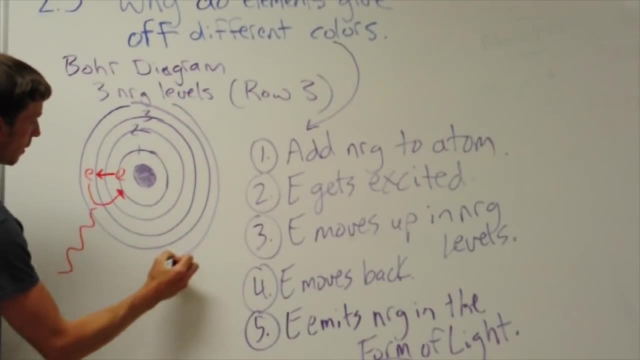 If it was going, let's just let's draw another energy level, let's kind of keep going with this. What if I had, you know, a couple extra? and you know, let's say that the electron I'm going to use just a black color just to indicate I'm going to move this electron, so no longer. 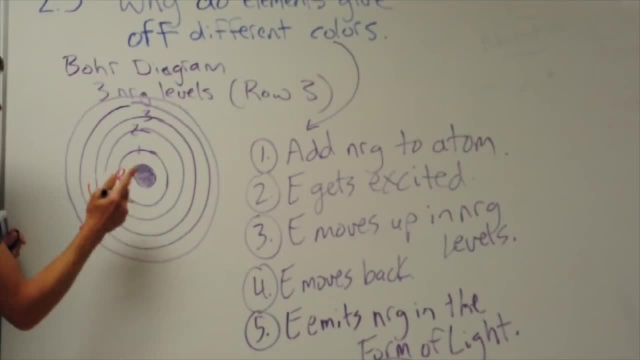 are we moving there right? We're going to take this electron and I'm just going to put an E now and let's move it all the way to energy level five. All right, So it's now here. So instead of the red color, it's at a higher energy level. 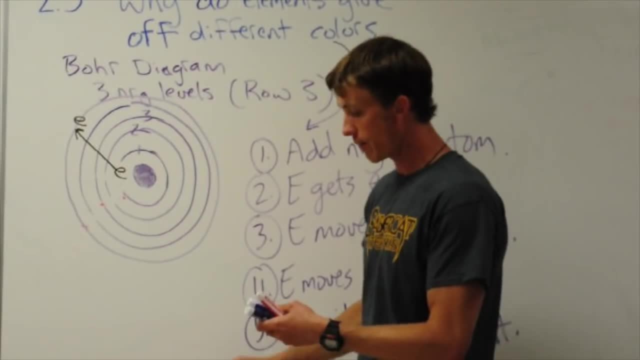 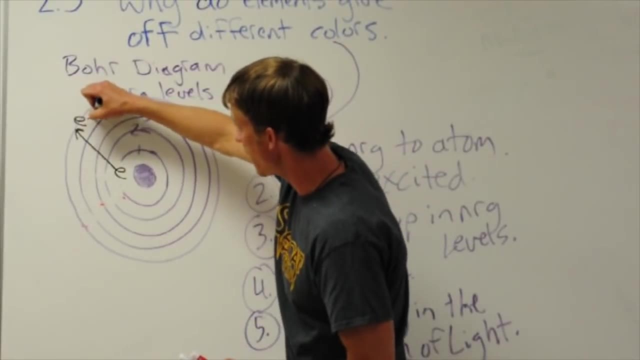 The electron itself is at a higher energy level, So it's going to go. it has to go all the way back. If it's going to go all the way back right after it gets excited, it's going to go all the way back. 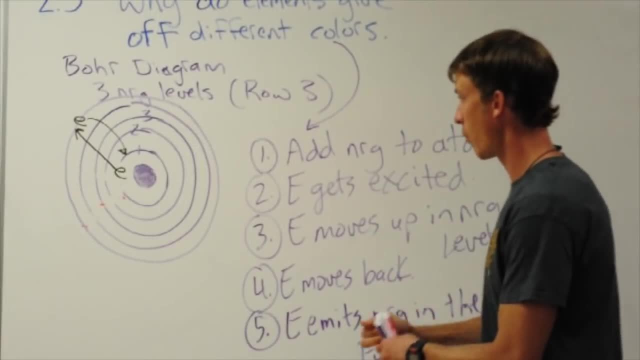 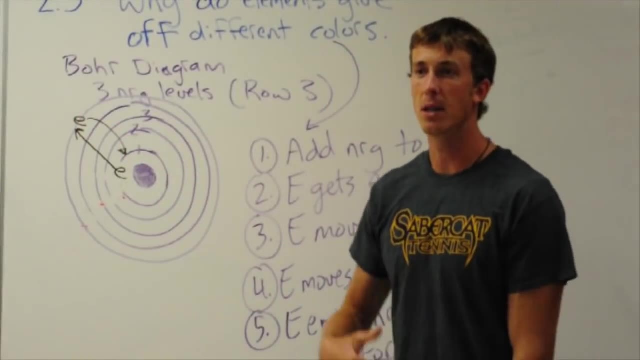 So it moves back, but now it's going to be an energy in the form of light. Well, what kind of energy is five energy levels compared to three? Well, if three was red, you'd expect five to be more energy, more frequency. 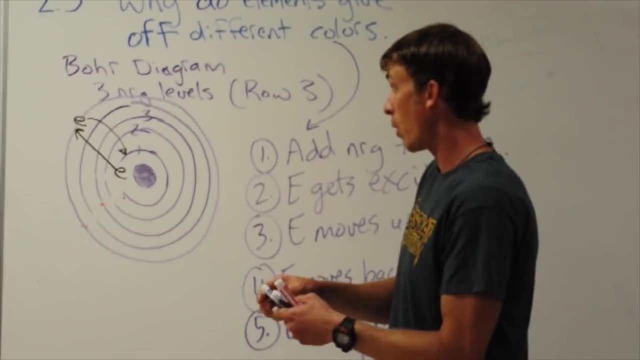 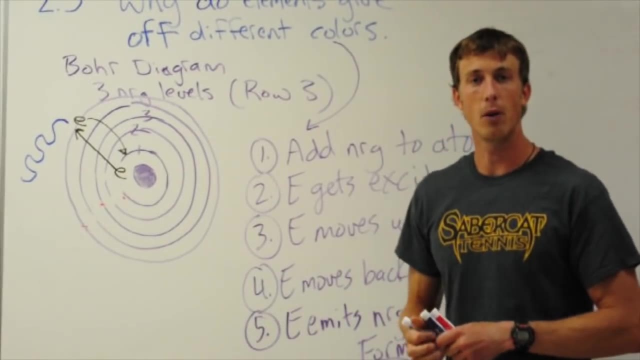 So you'd want a color, maybe that's a little darker, so maybe purple or blue. So let's just say it emits blue, so a little higher frequency, and it emits blue as the light. So it depends on where the electron goes in the energy levels.